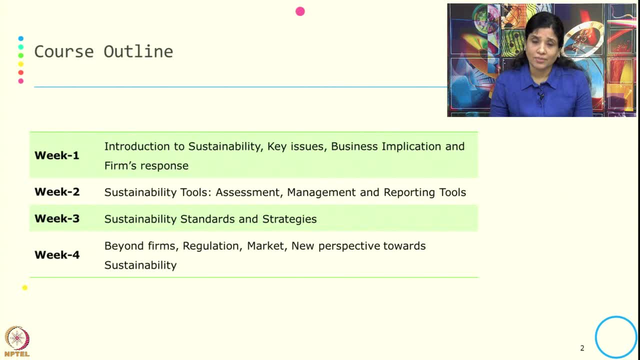 mostly we look at what are the startup, what is the role of the private sector in the sustainability. also, what are the new financial instrument that has come because of this sustainability And also at the end of it, we will try to bring a synthesis of whatever we have discussed in the sustainability. 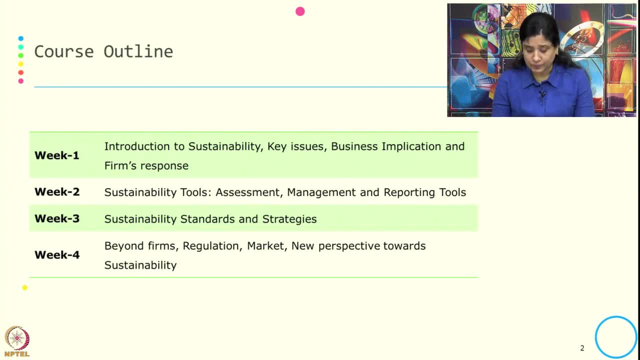 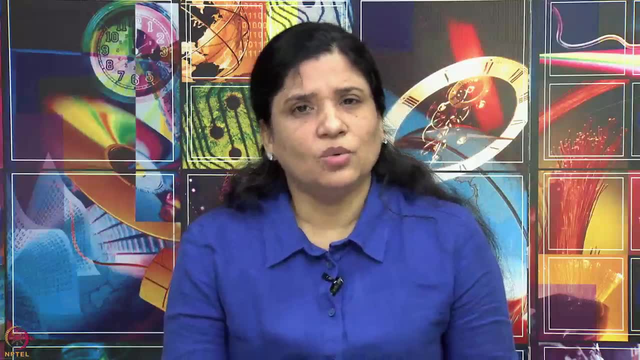 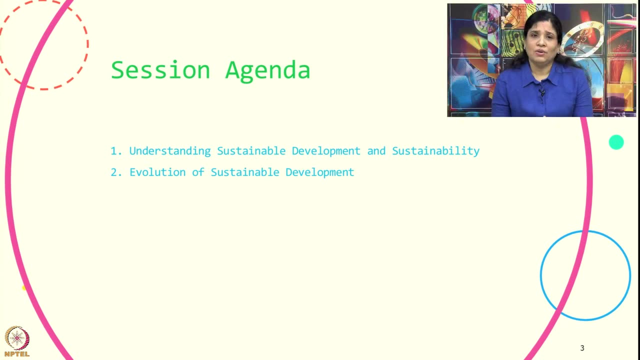 perspective. that is we are going we can add through this course. Now in this session, we will understand what is sustainable development, what is sustainability. Most of us, we know typically what is sustainable development or what is sustainability, but we will try to see how this. 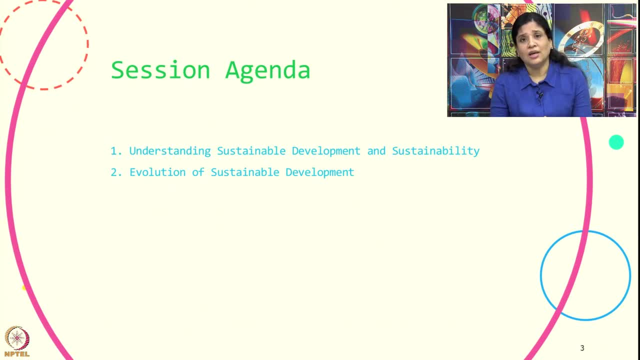 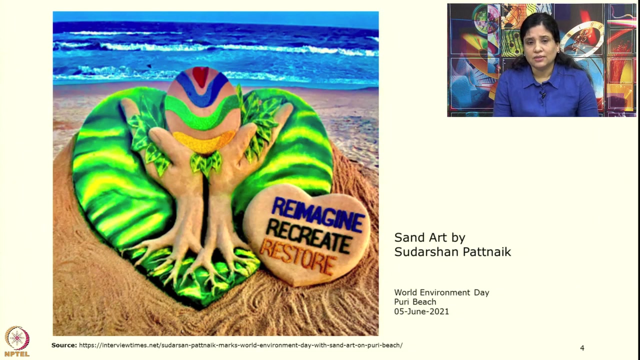 definition of sustainable development, what it was earlier and when it was widely accepted, and also we will try to see what are the different dimensions associated with the sustainability, And then we will see how the sustainable development that is evolve over a period of time. Now let me start this course with the, with a picture that was created 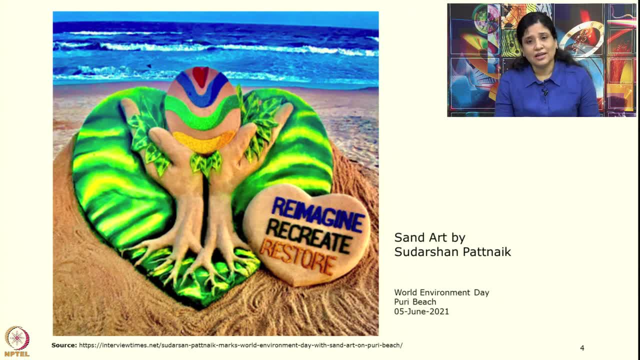 this is the picture of a sand art that is created by Sudarshan Patnaik, who we must be knowing. he is a sand art artist And he created this sand art in the pristine beach of Puri during the last world environment day, that is, in the fifth June 2021. 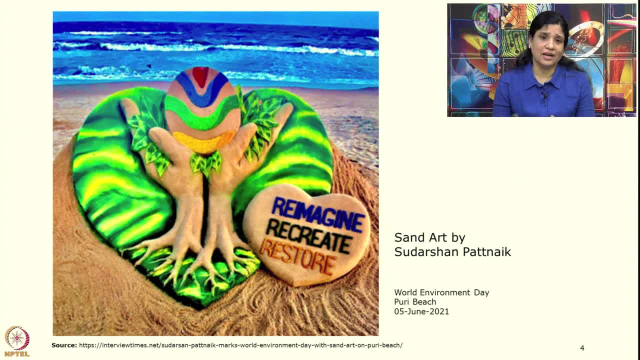 And the picture gives three words, that is, reimagine, recreate and restore. And the pictures speaks itself, and this is what the essence of this course, what we are going to deal with. It is all about sustainability, where we have to reimagine the 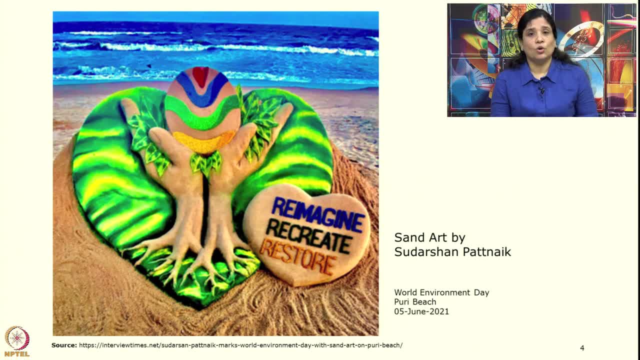 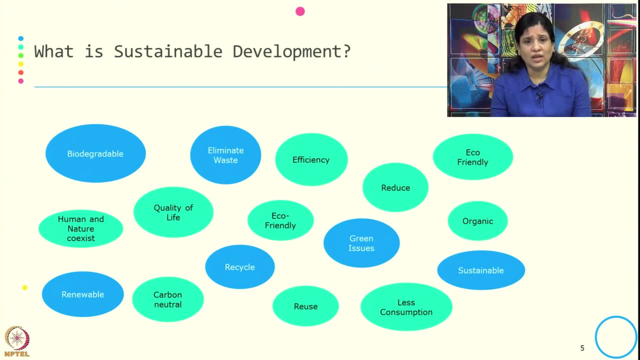 things, we have to recreate the things and we have to restore whatever we have damage or whatever. we Now coming to the fact that what we understand is the sustainable development. So if you ask anyone possibly the answer, what we get, someone just say that it may. 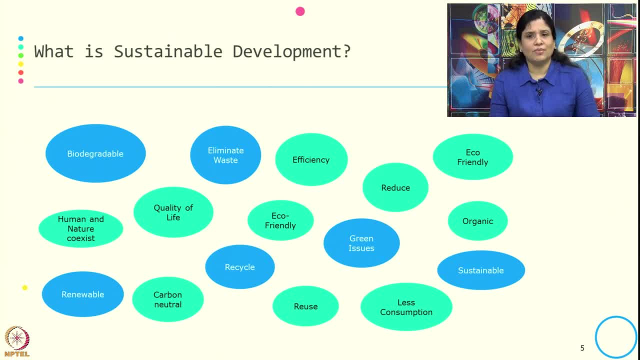 be eliminating waste. someone talks about quality of life. someone say: any eco-friendly, whatever is eco-friendly, environmental friendly, that is sustainable development. Someone says that the green issues related. those are sustainable development. some talks about carbon neutral, some talks about less consumption and I have picked up those words. 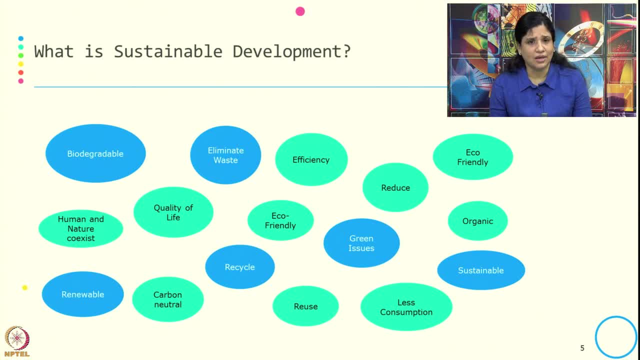 mostly from how we understand sustainable development. So more or less we understand what is sustainable development and we use the word what we feel that action can be over there or the agenda can be over there. So it like you take the example of your biodegradable or you take the example of your carbon neutral. 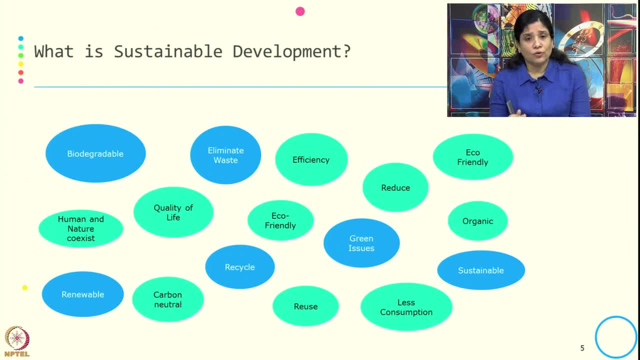 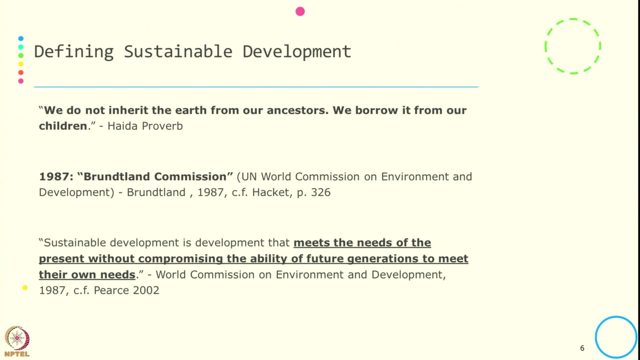 or renewable. So all these comes from the fact that what you feel, that the action is needed on this front or action is needed in the other front, and that is what typically the sustainable development is. Now let us see how we define the sustainable development or what are the formal definition. 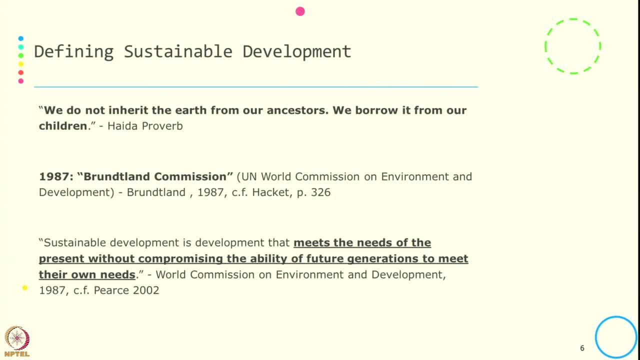 available for the sustainable development. So, the first one, this is a Haider proverb and this, this says that, or the, the way we define this, is that we do not inherit the earth from our ancestor. we borrow it from our children. And the widely accepted, or the popular definition, what for the sustainable development? it came. 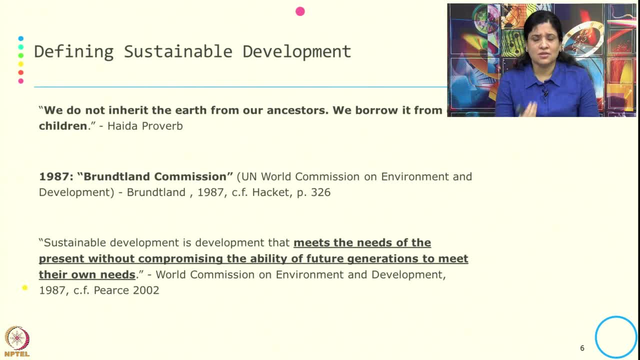 in 1987 from the Brundtland Commission. this is the UN World Commission on Environment and Development, And this says that sustainable development is the development that meet the needs of the present without compromising the ability of the environment. So this is the definition. 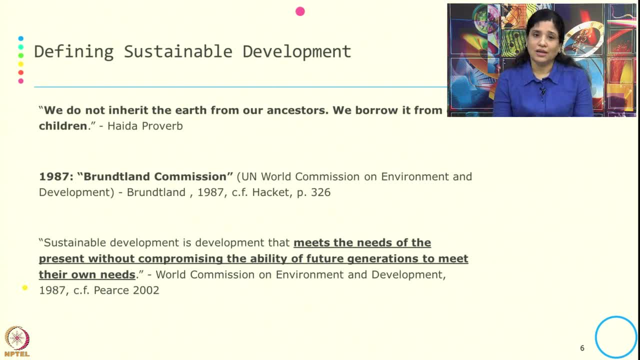 It is the ability of future generation to meet their own need, And so, till now, this is considered to be the most widely accepted definition of the sustainable development, where two things are being emphasized: one, the need- how we should meet the need. and second, it is not about only the present generation. also, it is about the 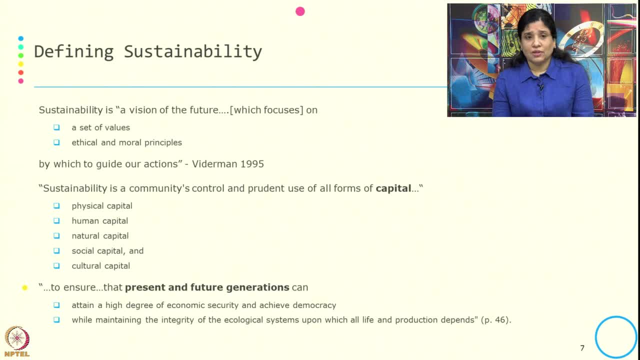 future generation. Now, going further, let us see how we define sustainability. So I have taken a definition of Weidman 1995 which says that sustainability is a vision of the future which focuses on two things. one, it is the set of values and second, it. 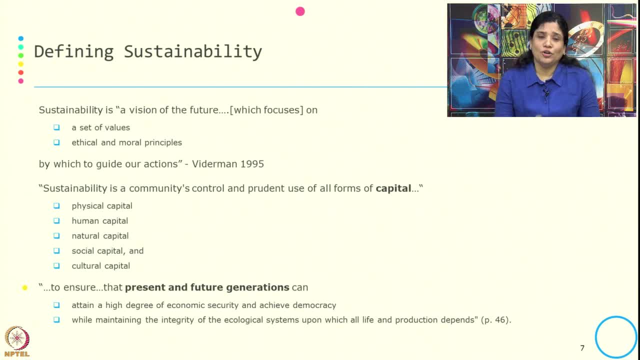 is ethical and moral principle. So at a later point of time we see that how, how? there is also an argument available from from an economist, that whether sustainability is ethical or whether sustainability is moral being, let us take this definition, which says that sustainability is a vision of the future. 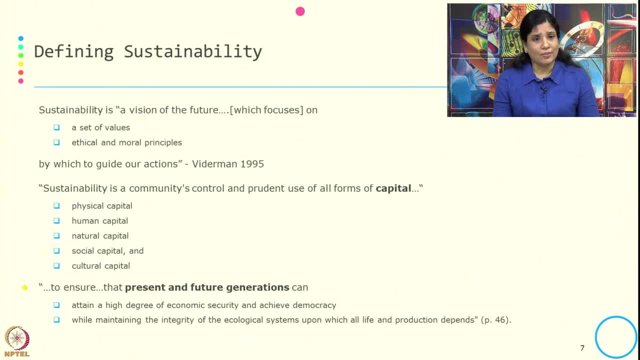 which focuses on set of values, ethical and moral principles, And this set of values and the ethical and moral principle by which to guide our actions. So mostly sustainability is all about our actions when it guided by a set of value and ethical and moral principle. 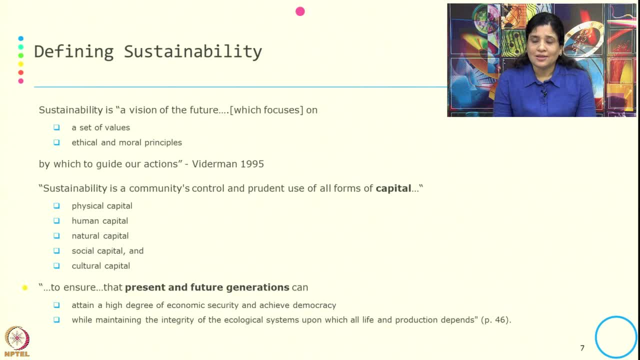 So by this now, what is sustainability? Sustainability is a community's control and prudent use of all form of capital. So now we are introducing the jargon that is capital and through which we are trying to understand what is sustainability. So sustainability is what? How the community controls the different form of capital. 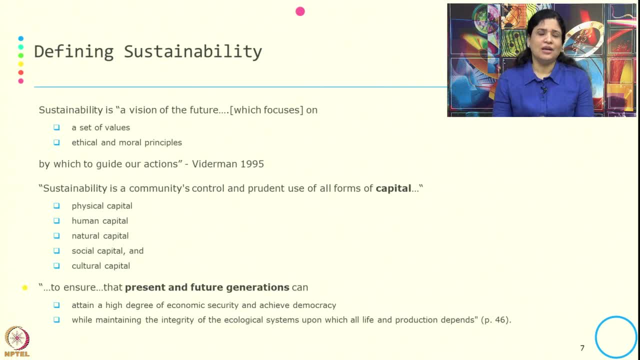 and how they do a prudent use of these forms of capital. that is a about sustainability. So there have been different types of capital, like physical capital, human capital, natural capital, social capital and cultural capital, And all this why there is a need for control and prudent use of all form of capital to 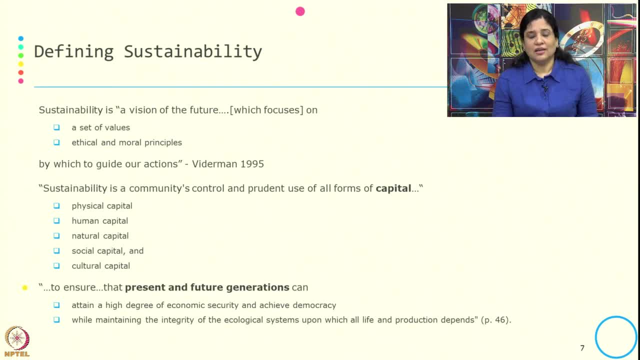 ensure that present and future generation can attain a high degree of economic security and achieve democracy. And by it is when they achieve the high degree of economic security and achieve democracy by maintaining the integrity of ecological system upon which all life and product depends on. So if you look at the entire slide, how we 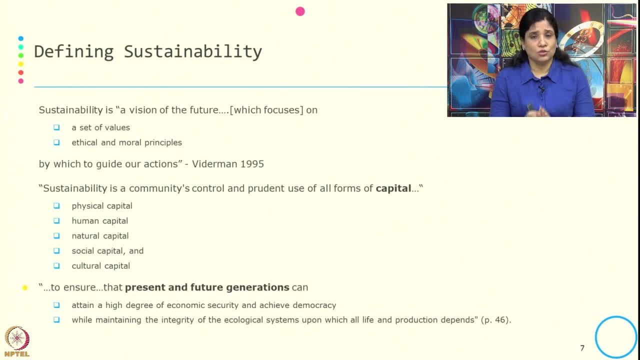 are trying to understand sustainability. Sustainability is mostly we need to. we are highlighting two things: One, how we should use the available capital, how we should use the available capital, how we should use the available capital, how we should control this, how we should use this, and this should be guided by the fact. 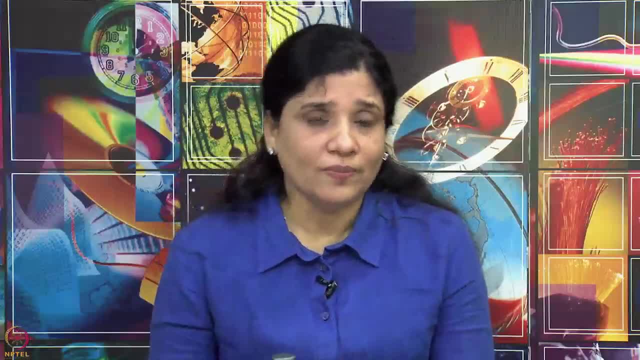 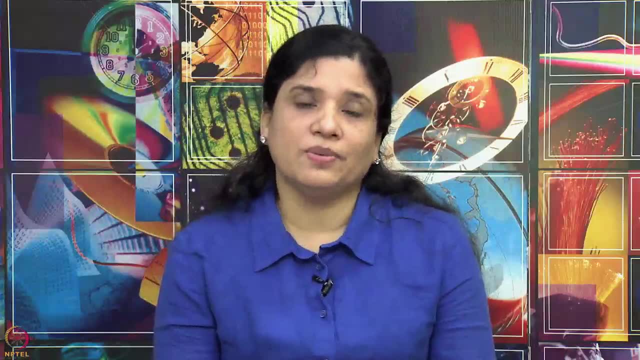 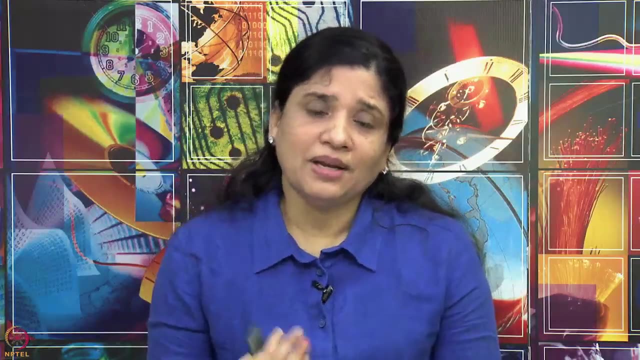 or the use or the control should be guided by a set of value and the ethical and moral principle. Now let us understand little bit more about the different types of capital which comes in the definition. Now, how do we define capital? Capital is typically- if you say this is the kind of inputs- right, it is a kind of a factor. 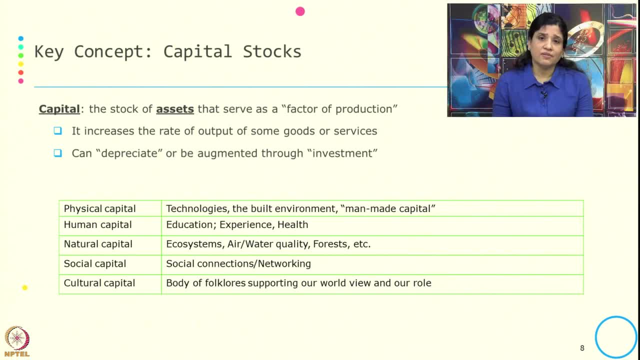 production. So capital is the stock of asset that serve as a factor of production. So it is one of the input in our production process. And what is the role of a capital? The role of a capital is that it increases the rate of output of goods and services. when we use this as the 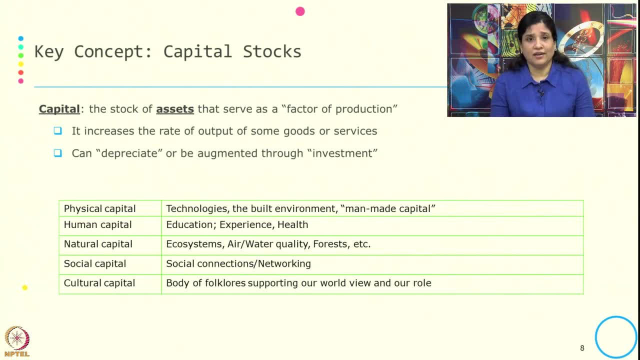 inputs and it can depreciate. this capital can depreciate over a period of time and it can be also augmented through the investment. So mostly capital is the input which is used in the production process. It may be used in the production process but it is not divided. 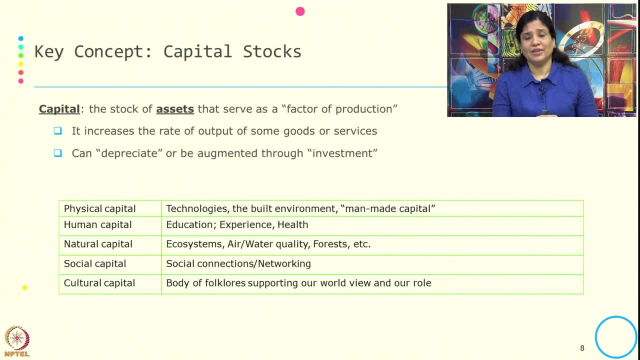 Capital is the stock of assets that serve as a factor of production. So it is one of the depreciate and it may augmented through the investment. Now let us see what are the different type of capital, what we have defined in the previous slide. So, in case of physical, 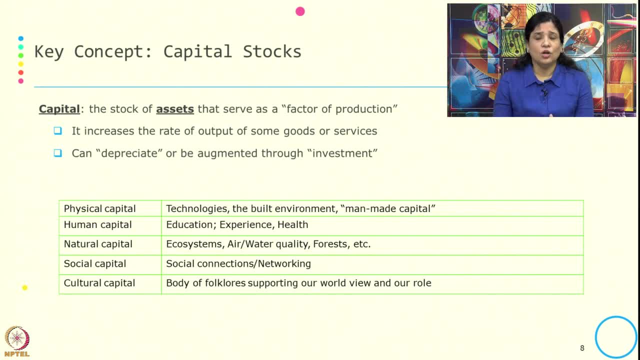 capital. typically we take the built environment, all the man-made capital, technology, the built environment, all this form of man-made capital that comes under the physical capital, Human capital, our education, typically the proxy of knowledge, what we get through our education, the experience of the experience, of working in the different fields, and also health. 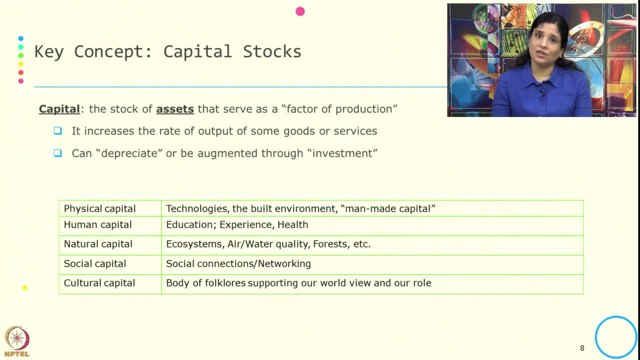 So these are the three main thing: what we take in the in the context of the human capital- education, experience and health. Then we take the natural capital, and the natural capital we take all ecosystem resources- air, water, quality, forest- So it includes everything. 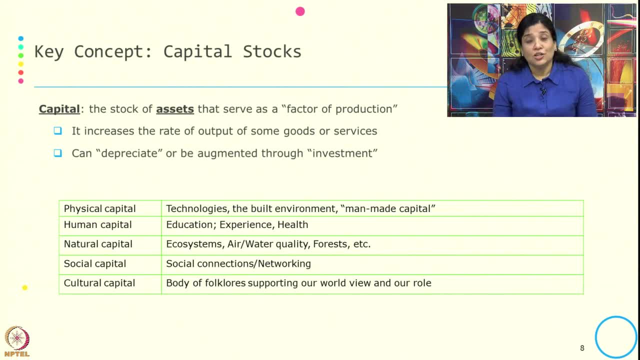 that we have defined in the previous slide. So it includes everything that we have defined in the whatever comes under the ecosystem resources, Social capital, where we take the proxy for our social capital, when we take the variable, for this is social connection, social networking, 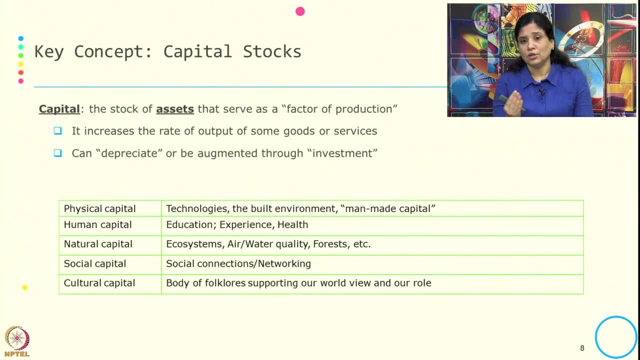 And cultural capital is the body of folklore supporting our world view and our role. that comes under the cultural capital. So some point of time it is easy to operationalize what comes under the physical capital, human capital and natural capital. But it may be little indirect when it comes to the social capital and the cultural 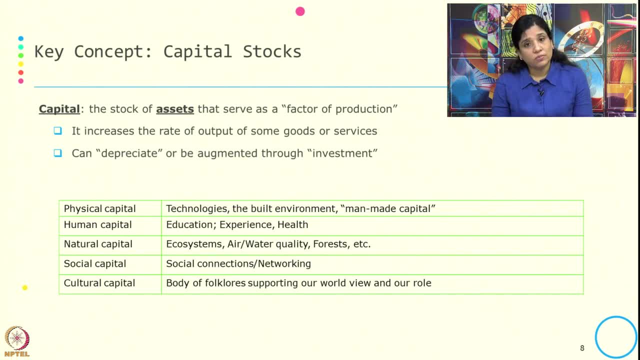 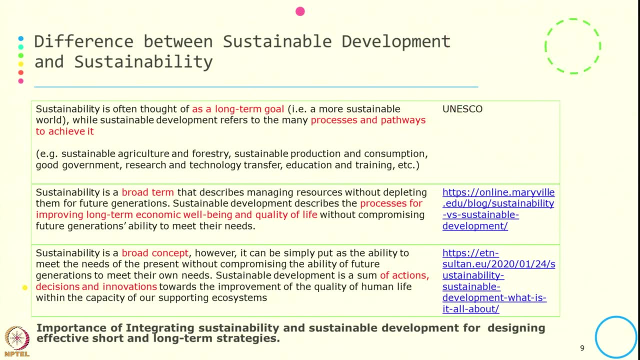 capital, but they do play a role in our operationalizing the sustainability. Now, many times you, many times you must have heard that we use the word sustainability and sustainable development interchangeably, right? So sometimes we say it is sustainable development, sometimes we say sustainability. So explain to us that. what is the meaning of the term sustainability? 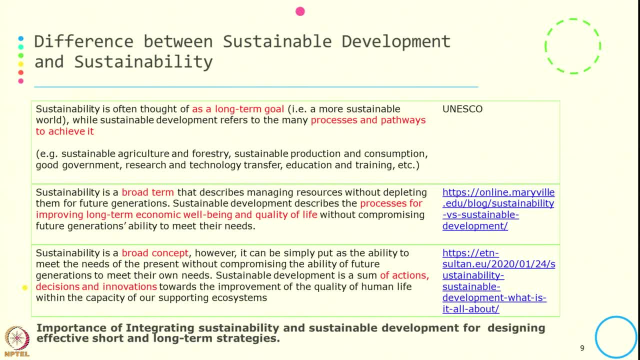 So there are difference between sustainable development and sustainability. Some point of time it looks very finer, but we go in depth. there is a significant difference between the sustainable development and sustainability. Now I have picked a few differences that have been cited by a different in the different. 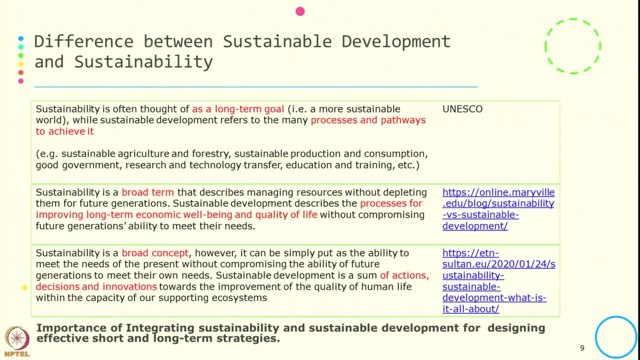 vlog or the different site and we will see what, how they define or how they differentiate, the differentiate between sustainable development and sustainability. So the first one is from UNESCO and here the way they brought the difference is sustainability is often thought as a long term goal, that is, more sustainable world and sustainable. 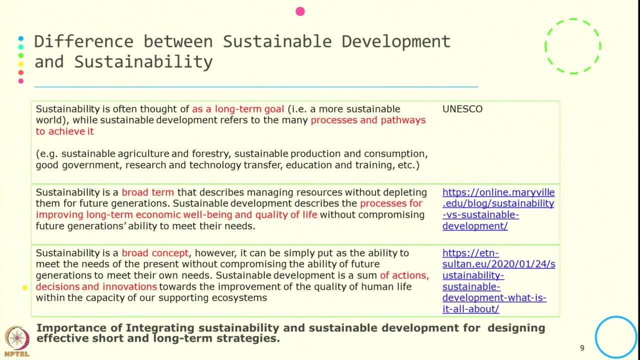 development refers to many processes and pathway to achieve it. So sustainability, development, sustainability is a long term goal, mostly when talking about a sustainable world in next 20 years, then 30 years, then becomes the or 50 years. that is sustainability, but sustainable development talks more about the processes and the pathway. 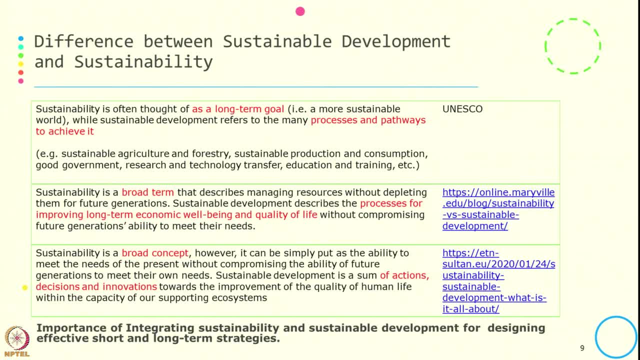 So the typical example of processes and pathway over here is that when we say that we are adopting a sustainable agriculture or sustainable forestry, or we are talking about sustainable production, consumption, good government, research and technology transfer, education and training, So these are all this comes under the process and the pathway. 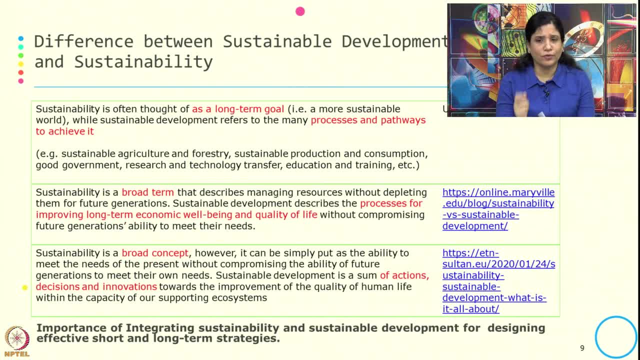 The second one is from a blog by blog, from Maryville, and how they have define or how they have identified the difference between these two terms. So, for them, sustainability is a broad term that describes managing resources without depleting them for the future generation. 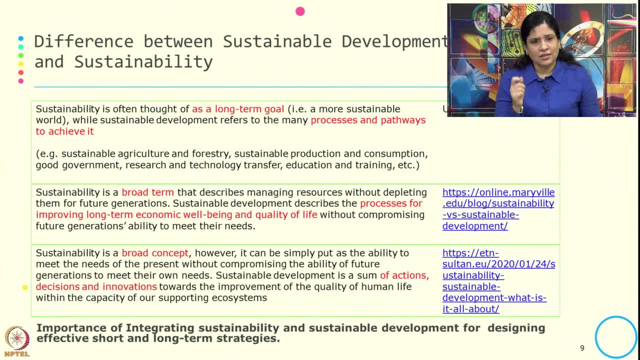 So it is a broadly they say that sustainability, where we are managing the resources without depleting them for the future generation and how they have, define sustainable development. that is the process for improving long term economic well being and quality of life without compromising the future generation ability to meet their need. 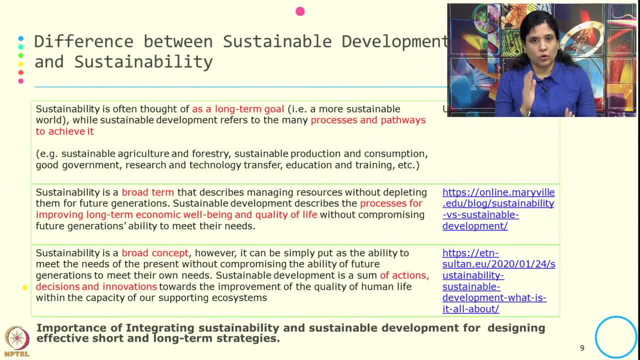 So the difference over here is that one is it is a broad term, about managing resources, and second is about this is a process for improving the long term economic well being without compromising the future generation ability to meet the need. So here also the difference is one is a broader term and second, one is getting into the process. 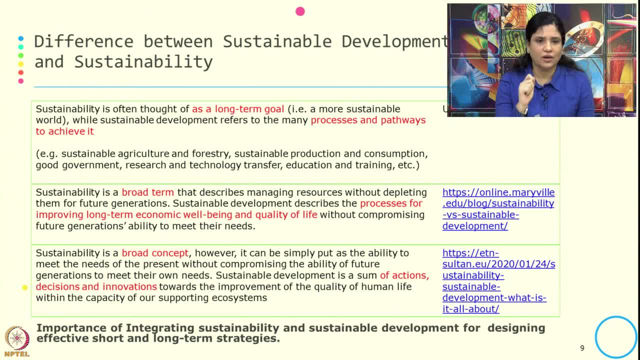 If you come to the third difference, or the third kind of difference, what I have picked up- this is also from another blog, which says that sustainability is a broad concept but, however, it can be simply put as the ability to meet the need of the present without compromising. 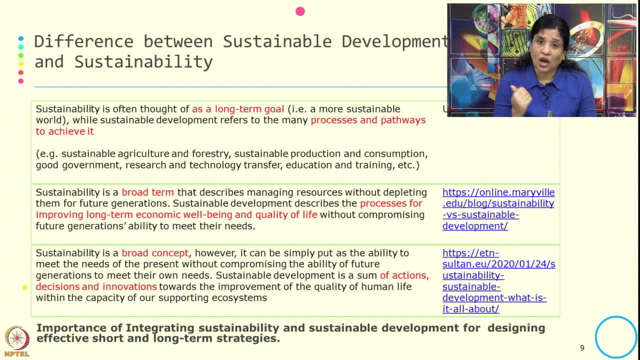 the ability of the future generation. And how is the sustainable development? It is a sum of action, decision, innovation towards improving the quality of human life within the capacity of supporting ecosystem. So, mostly from these three opinion, what we have taken about the difference between sustainable 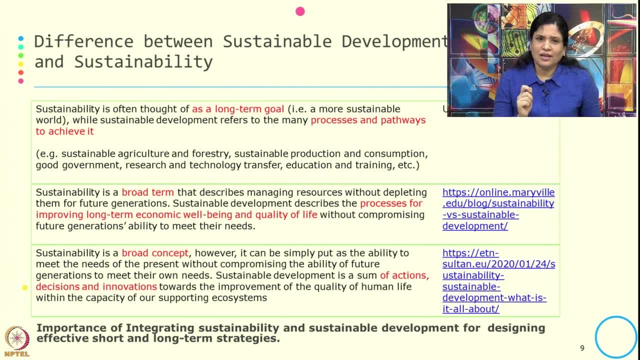 development and sustainability. if you see, in every case, sustainability is more about a broad term, broad concept, Long term goal, and sustainable development is more about process, pathway, actions, decision and innovation. But what is important is that we need to integrate this sustainability and sustainable development. 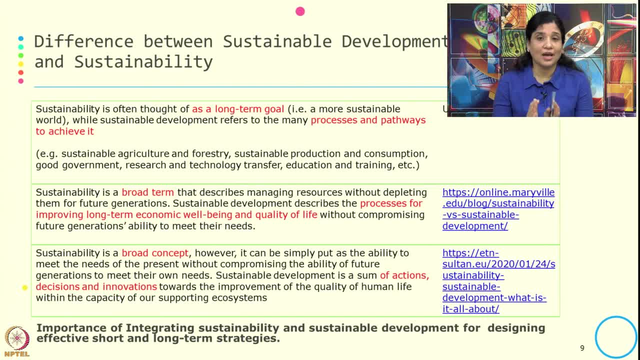 for design the effective and effective short term and long term strategy. So possibly mostly one of it is goal broad concept. Second one is the process, Second one is the action, But the integration of both needed when we are designing the short term and long term. 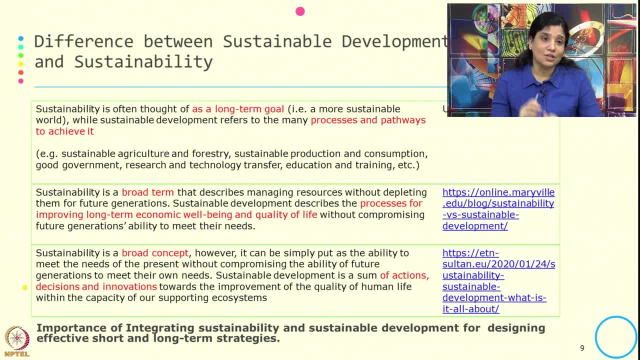 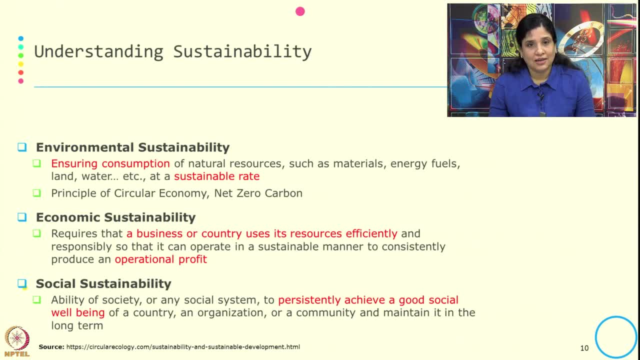 strategy, then only it would. we can see the so called sustainable world. Now let us understand sustainability more by understanding what is the dimension associated with the sustainability. So there are mostly three dimension of sustainability. One is environmental sustainability. Second one is sustainability. 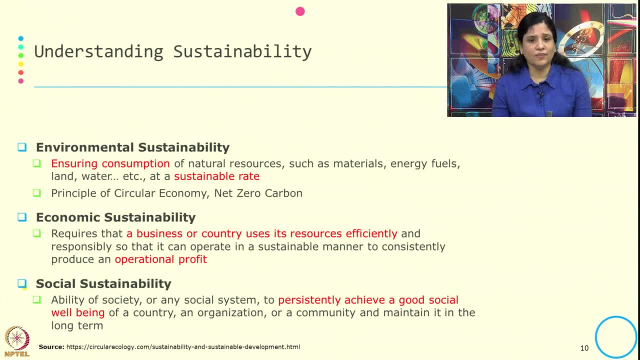 Second one is the economic sustainability And third one is the social sustainability. Now, what is environmental sustainability Here? typically, we ensure that the consumption of natural resources such as material, energy, fuel, land, water should be at a sustainable rate. So mostly we are ensuring a sustainable rate of consumption in case of environmental sustainability. 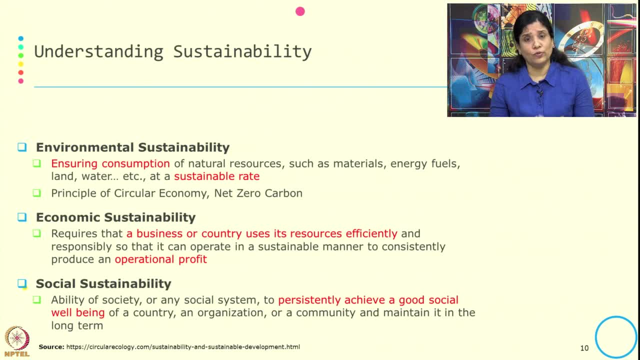 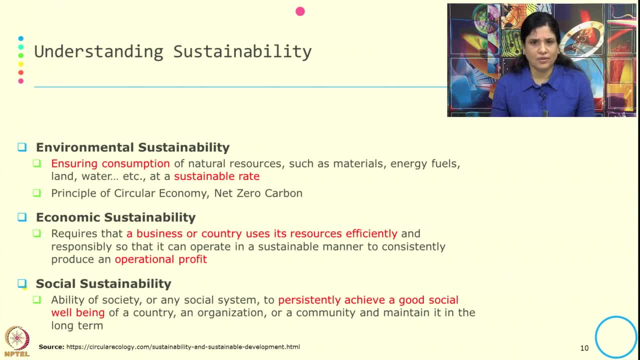 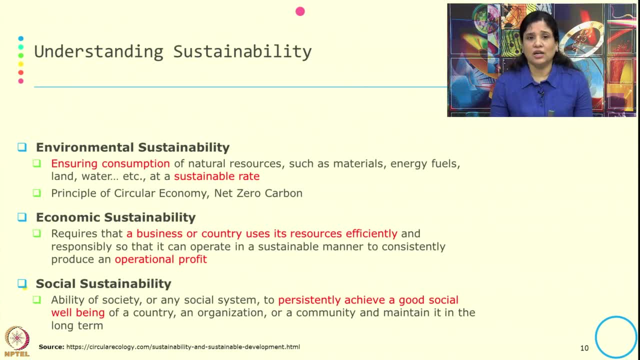 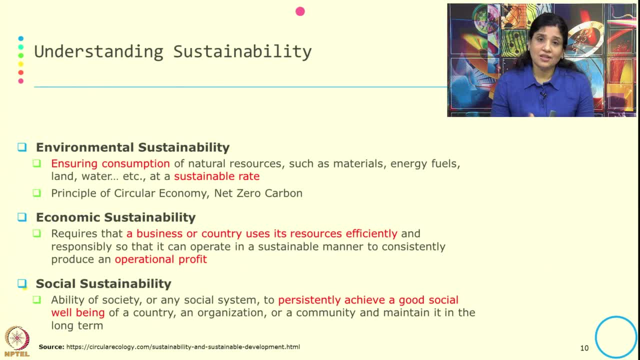 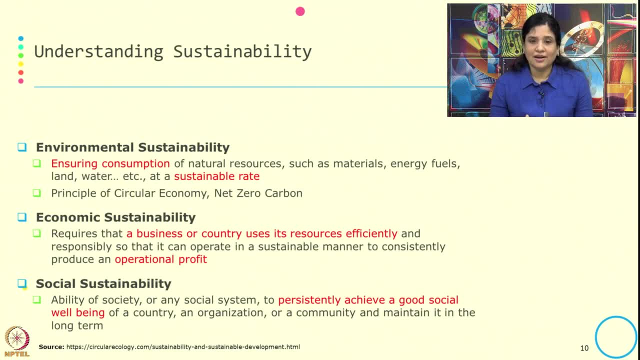 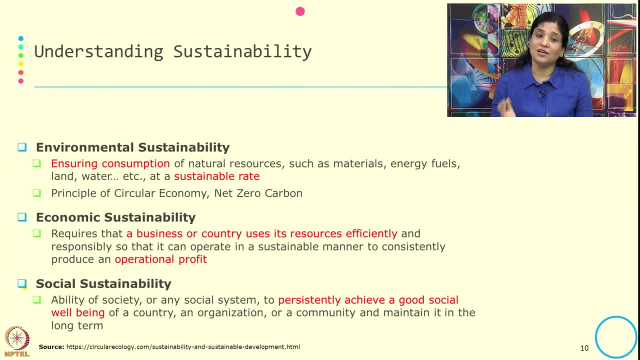 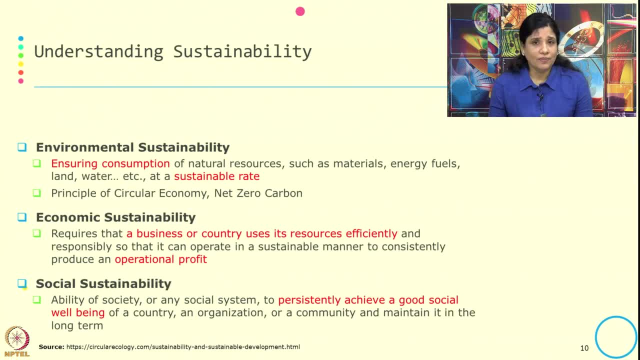 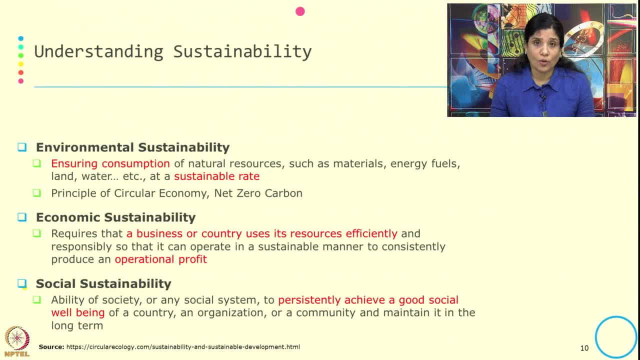 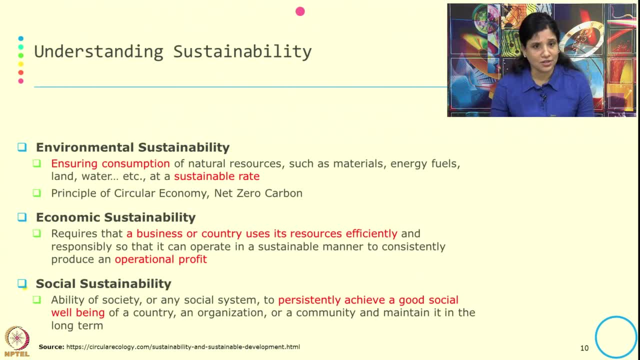 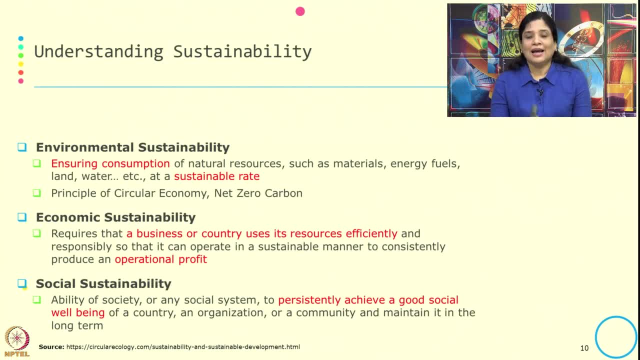 So, let us start, So let us start, So let us start. The last dimension, or the third dimension of sustainability is social sustainability. So what is social sustainability? Ability of society or any social system to persistently achieve a good social well-being of a country, of an organization or a community, or maintain in the 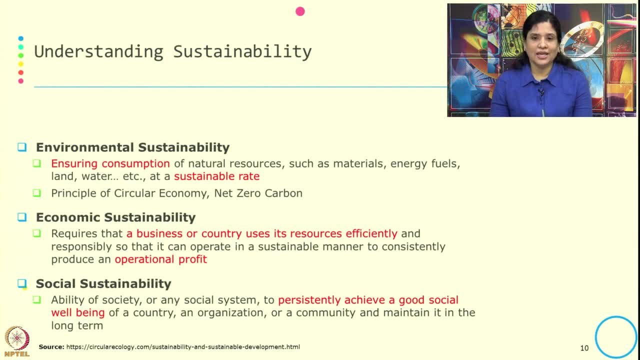 long run. So social sustainability is what It is about: achieving the good social well-being for the in different scale, like in a community, like in an organization or in the country as a whole. And also one is achieving the social well-being and second is to maintain it in the 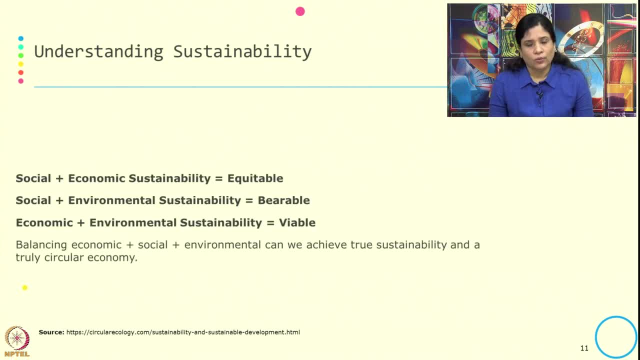 long term. Now, when we are talking about this three dimension of this sustainability, that is, social, economic and environmental sustainability. Now, what we achieve when we maintain the social well-being Ability of society or any social system to persistently achieve a good social well-being Ability of society or any social well-being Ability of society or any social 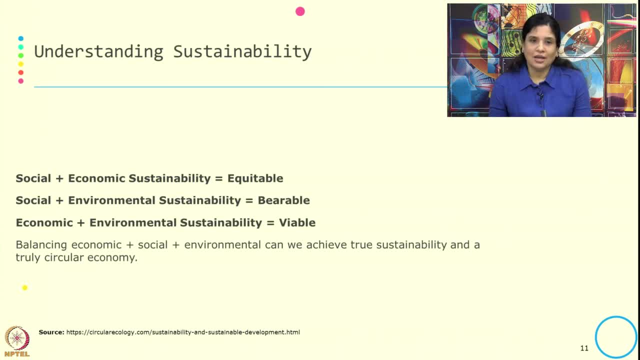 well-being, Ability of society or any social system to persistently achieve a good social well-being, This sustainability. So when we maintain social and economic sustainability, possibly equity, the equitable is the achievement. When social and environmental sustainability, it is about variable. 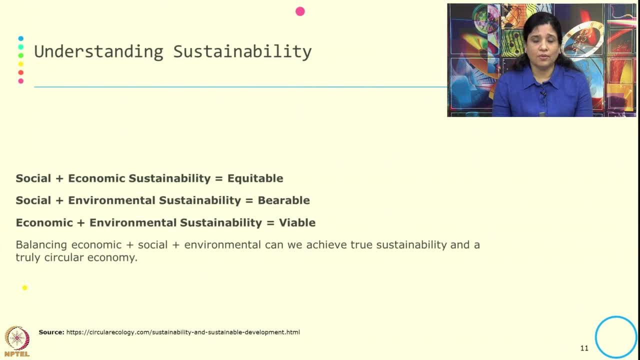 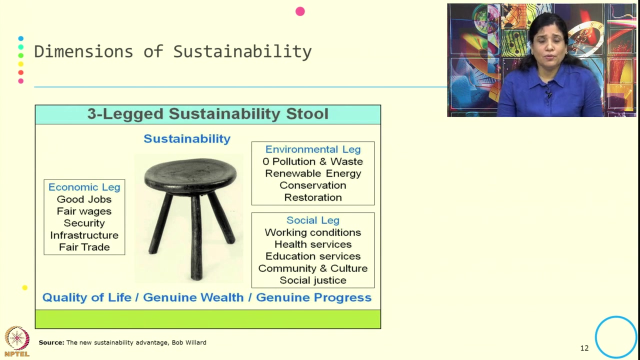 and when economic and environmental sustainability, it is viable. But the what is most important over here is that we need to balance economic, social and environmental. then only we can achieve the true sustainability and true circular economy. ok, Now this three dimension of sustainability is beautifully explained through a three-leg. 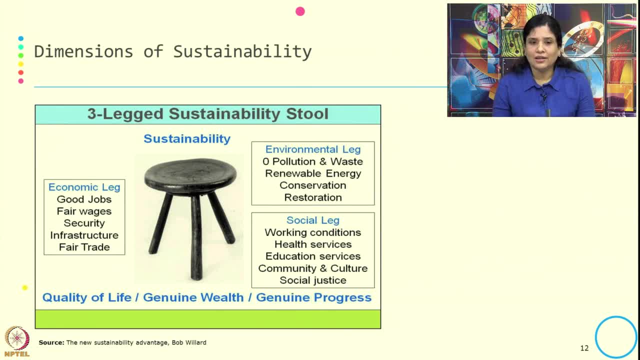 sustainability tool in the by Bob Willard in the in his book New Sustainability Advantage. So this three dimension is considered as the one or three legs of this sustainability tool And here, if you look at, there is a economic leg, there is a environmental leg and there is a 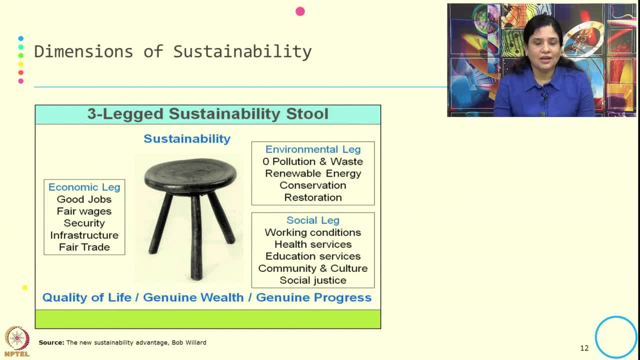 social leg. So in case of economic leg, you find typical indicator of economic leg is: good job, fair wages, security, infrastructure, fair trade. all this comes under the economic leg. Environmental leg it is. it includes a zero pollution and waste. 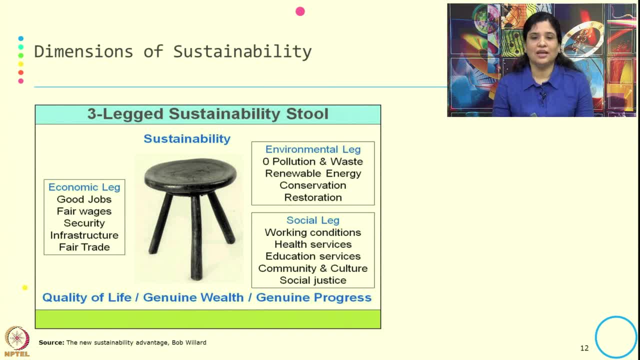 renewable energy, conservation, restoration- And social leg is how we are performing in term of working condition, health services, education services, community culture. what is the status of the social justice? So this entire three dimension is understood through this three different leg, and each leg consist of those indicators which 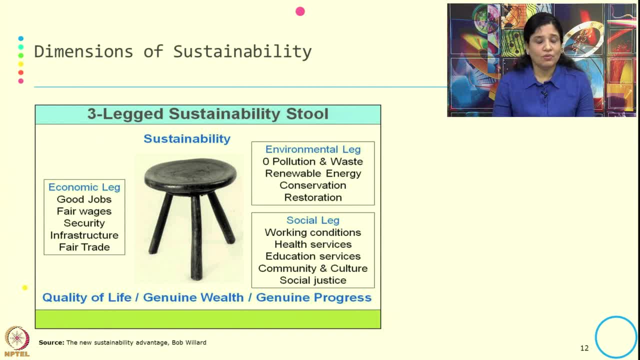 represents the economic well-being, environmental well-being and social well-being And, at the end of it, what we get? We get the better quality of life, genuine wealth and genuine progress. That is the end outcome when we are doing well in all these three dimension. that is economic. 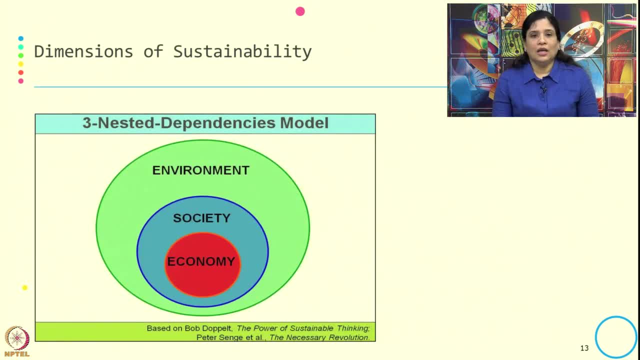 environmental, social. Now this dimension of sustainability, if you look at this, is again explained through the Nestor dependency model And all these three indicator. in fact, they are dependent on each other. So society is dependent on environment, economy is dependent on society. So in a bigger scale, it is environment a subset. 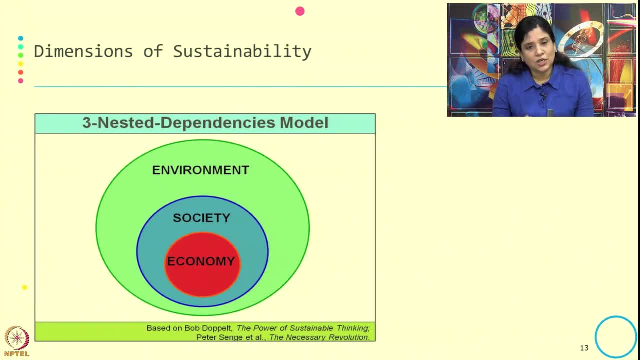 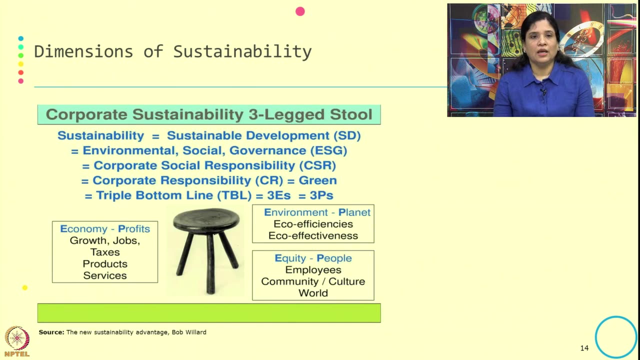 within that environment is society and subset within the society is our economy, And all these three are interrelated. possibly they will not be able to function if they are not dependent on each other. Now, little bit extending more on this sustainability, that is mostly in the context of corporate sustainability, that how, this three 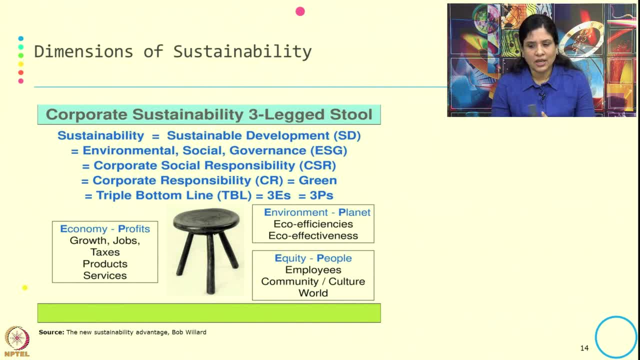 dimensions are explained further, So must be hearing the different jargon those are being used these days. So, as I have said, these three are interrelated and the it has certain different limits and kind of. we will discuss about how these three are interrelated and interrelated And we 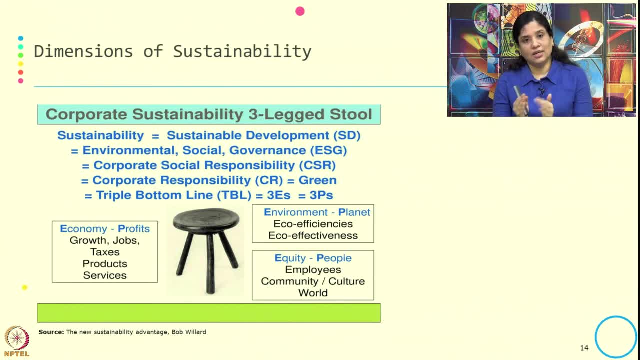 So possibly we discuss about sustainability. what is sustainability, what is sustainable development? but the newest jargon, or the different jargon over a period of time, what we keep hearing is that ESG, that is, ESG investment, ESG reporting, so which says that environment. 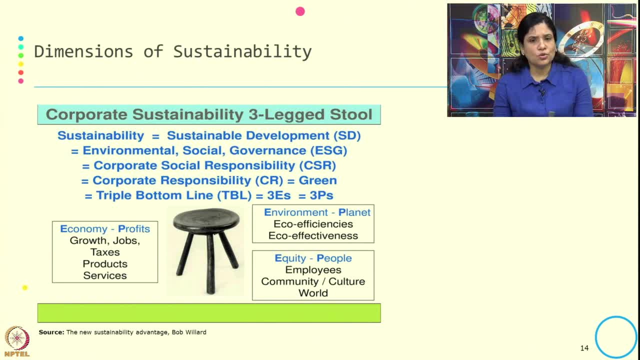 social and governance, then CSR, that is corporate social responsibility, then CR, that is corporate responsibility, then green triple bottom line. three E's, three P's- these are all the jargon those are being used and but the end of it, what it calls that these are all. 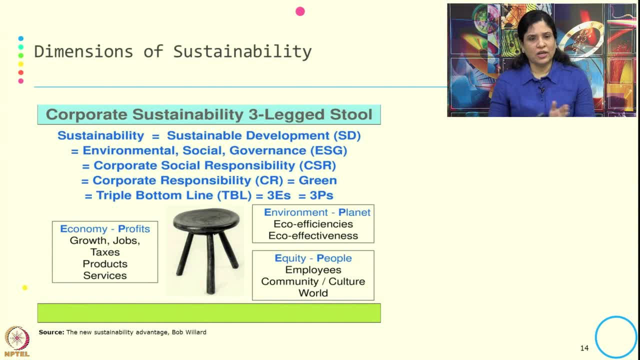 sustainability. So it is when you say environment, social governance. here also they are trying to say that how you achieve the sustainability, or how we should use what is our corporate social responsibility and how we should use this to achieve the sustainability. Similarly, corporate social responsibility, then corporate social sustainability, then. 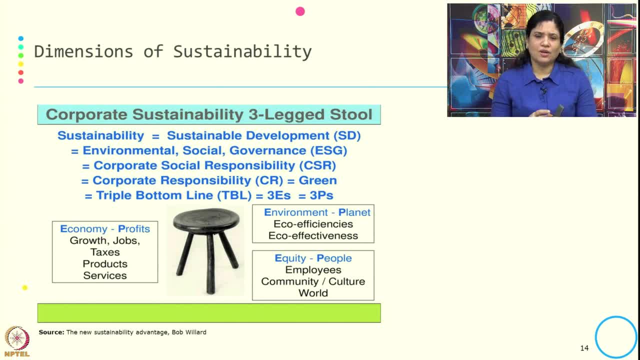 social responsibility, all these green triple bottom line, at the end of it the achievement, what we get, that is the sustainability. So again bringing this three dimension is that when we say three E's or three P, so when we say three E's, that is economic, environment and equity. when we say three P's, this is. 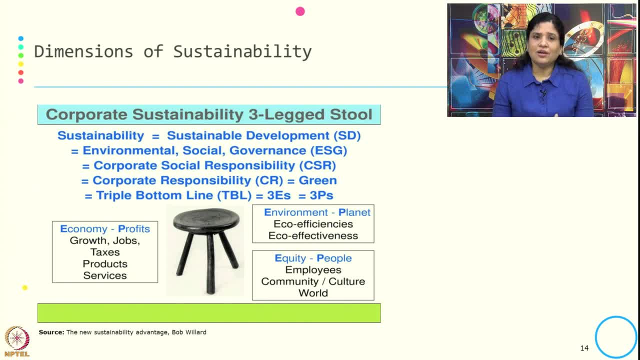 profit, planet and paper, And what are the indicator or what are the variables associated with each of it? When we say economy and profit, typically it is about economic growth, mostly all form of economic growth, jobs- that is the indicator of employment, taxes, products, services available. 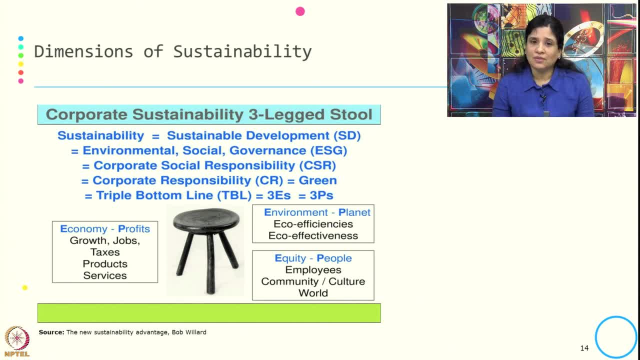 in the market. When you talk about the second E and second P, that is environment and planet, that is eco efficiency, eco effectiveness that brings the variables for the environment and the planet. And in the third one, when we talk about the third E or third P, that is equity and people. 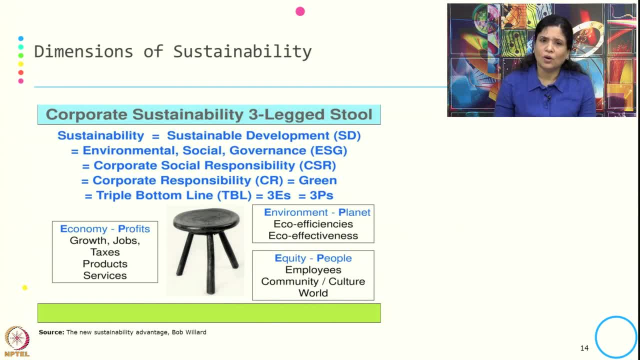 and that is employees, community culture, all these thing that comes under the third E and third P. So mostly the sustainability is about the three E's, that is, economic, environment and equity Economy is representing the economic part of sustainability. environment is representing 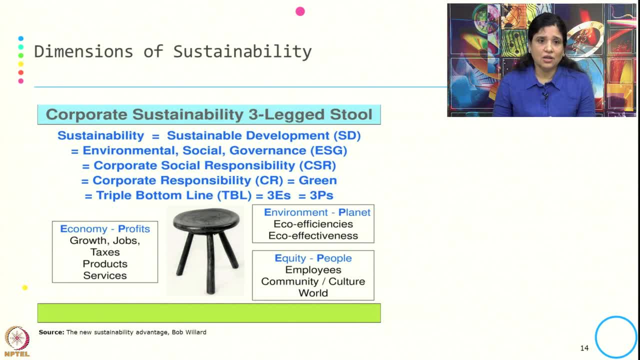 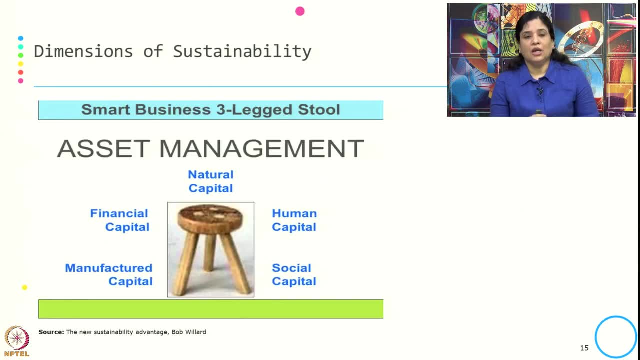 the environment part of sustainability, and equity is representing the social part of the sustainability. Now let us see how this different form of capital is again explained through this so called sustainability tool. So, if you remember, when we are trying to define sustainability, we said that this is: 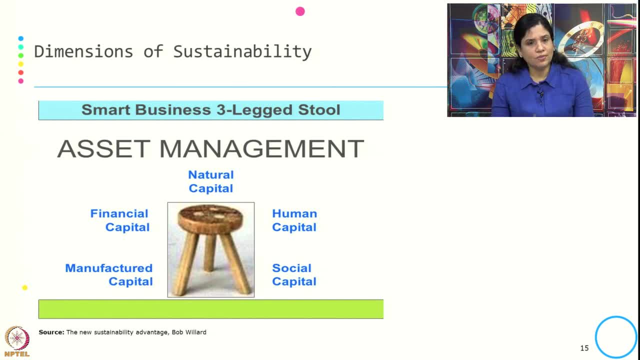 the control and prudent use of all forms of capital. So here, how this being managed. so, at the end of it, whether you follow a model of 3E, whether you follow a model of 3P, it is end of end of the day. it is about how do you manage.